so if you have your website images loading horribly like this, where you just wait so long for the image to load and sometimes you get like blank spaces in here and the image does actually take forever to load and the user experience is just awful out of the box, like the user can't tell. 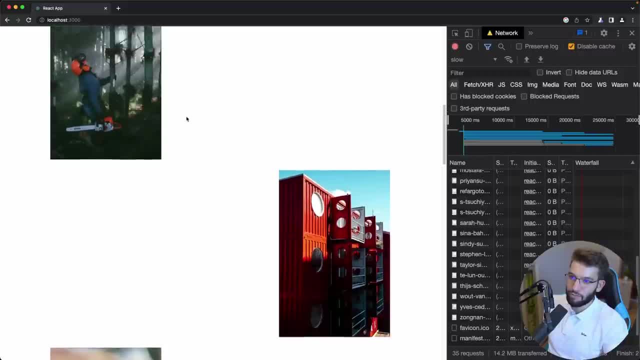 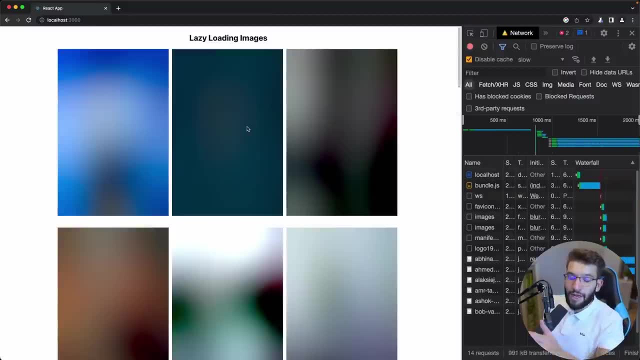 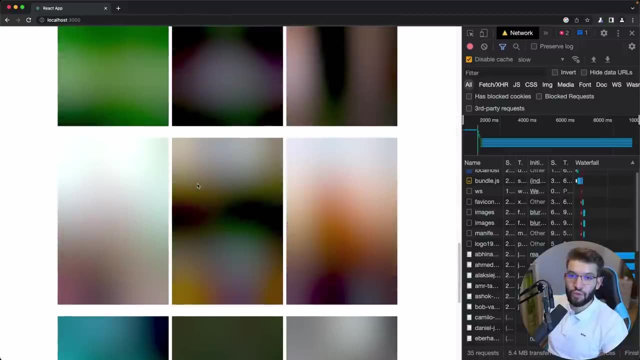 if the image is loaded or not. you got image loaded here, not like on the top, and here it's not loaded yet. it's crazy and it's very, very bad, where, in the other hand, you can have it loading like this with really awesome placeholders in here, and it tells exactly the user what the image would look like. 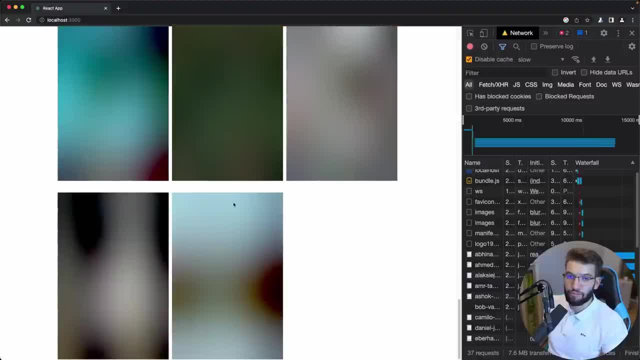 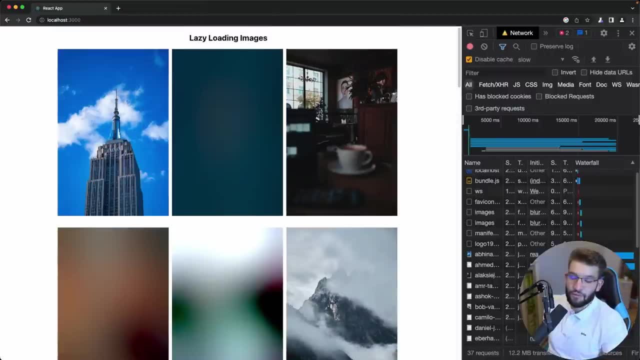 with a really awesome kind of like blurred version of the image before it actually loads, of course, because we're using some slow network in here to throttle the network and once the image is fully loaded, you're going to see that image showing up instead of the placeholder. it's just an amazing. 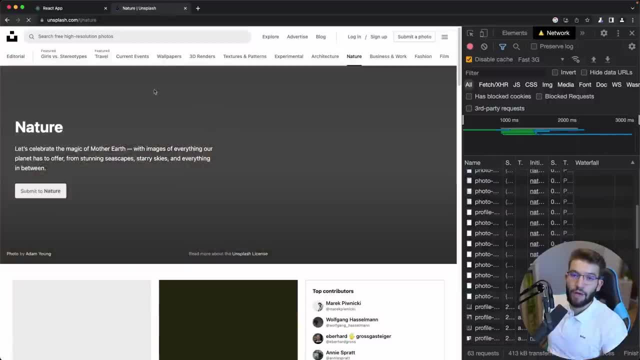 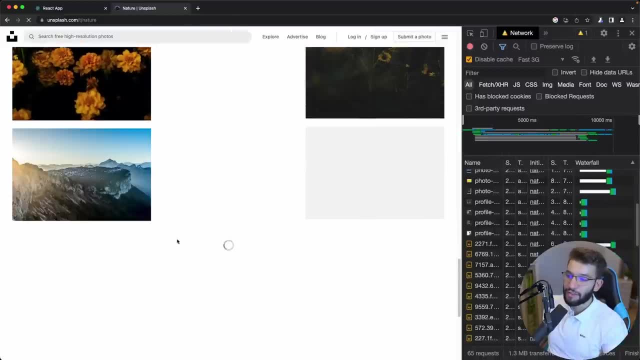 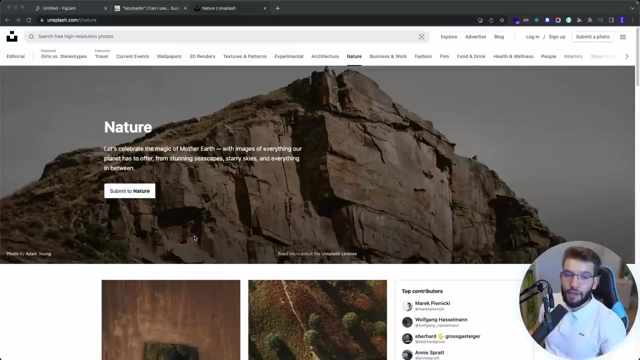 user experience, and that's the same awesome experience that insplash provides when it comes to loading images, with this really awesome placeholders and blurred version, of course, it lets you see what's going on with the image without looking at it. so if you want to check out a video on how to load images in just one second or two seconds and, of course, lazy loading- 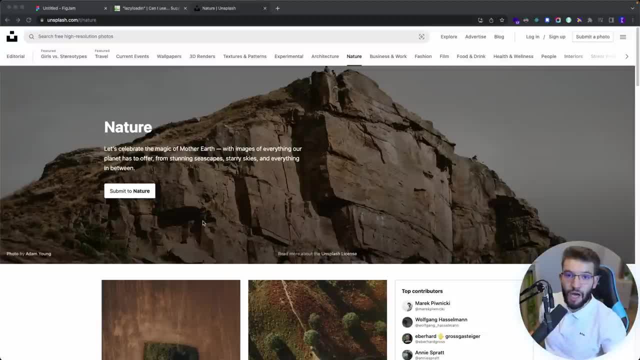 the images once the user reaches the bottom. so image optimization is very, very important in the web standards or in a browser in general, so as, as web developers, we need to optimize our images in order to be had better, have like a developer experience and as well, of course, we care about. 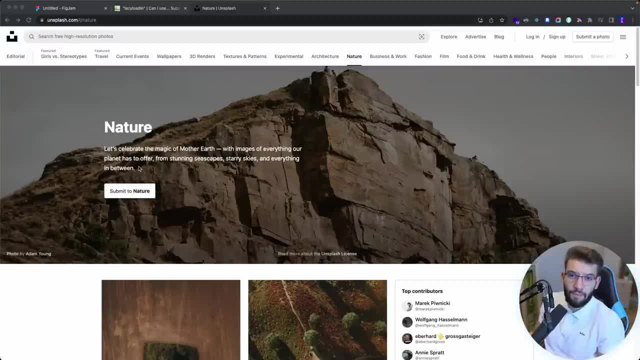 a lot about the user experience and the page load time. so that's what i was struggling with and when images like 4K and 8K, I was struggling to load all of those And I was looking and digging deeper into how to better optimize this and what are the best ways. 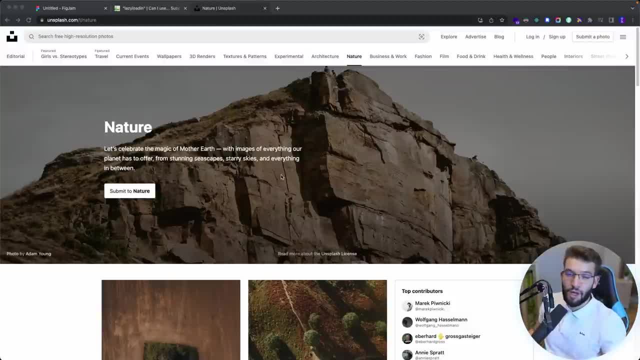 And one of the best ways, obviously, is lazy loading images. And what I mean by lazy loading images actually only load the images when the user scrolls into that image, So if the actual image isn't in the viewport, like in Splash, 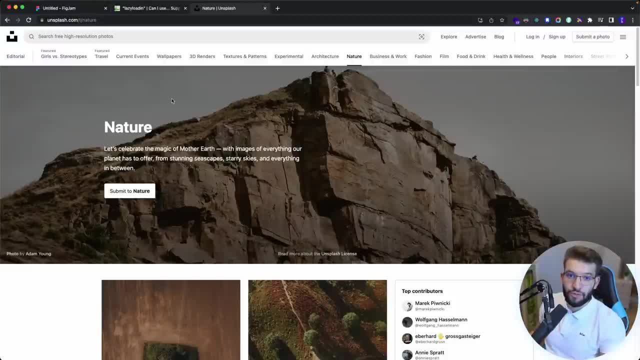 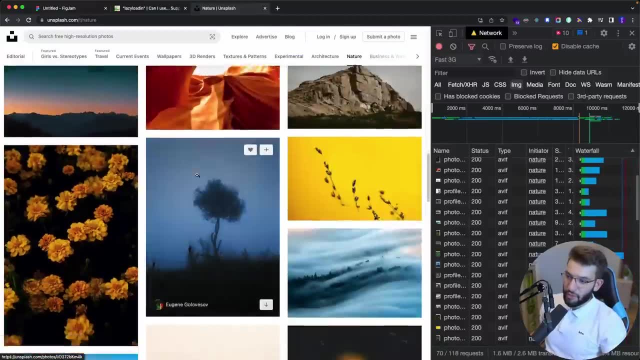 as we all know, Splash is a great, great website that offers really awesome experience. So I seriously added some network fraud in here And some images are not loaded. It shows you some really nice placeholder And if I scroll down, some images are not loaded. 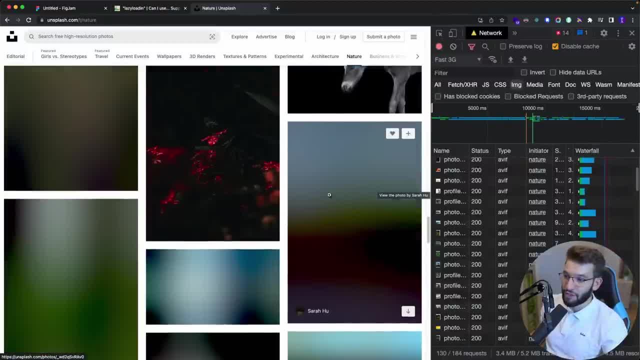 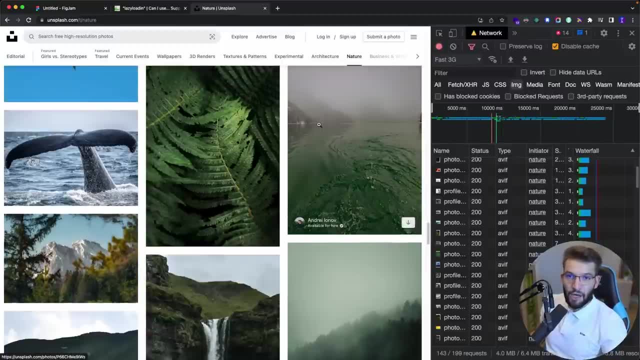 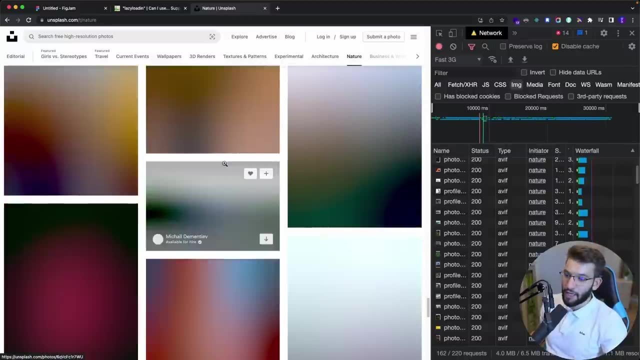 And it just keeps showing you this placeholder into the image is actually fully loaded And this is absolutely an awesome experience because it gives you this really awesome placeholder that can tell what exactly the image would look like just from looking at blurred placeholder thing, which is not going to take that much, obviously. 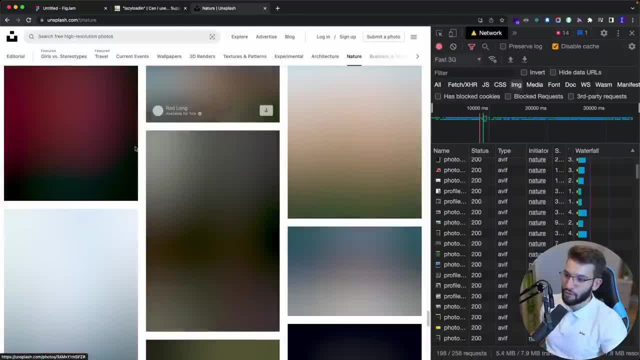 So if you look at it, it's crazy good And it's super, super fast to look at all these images. And that's what lazy loading is. It's blank in here, but it just go ahead and fetches all the images. 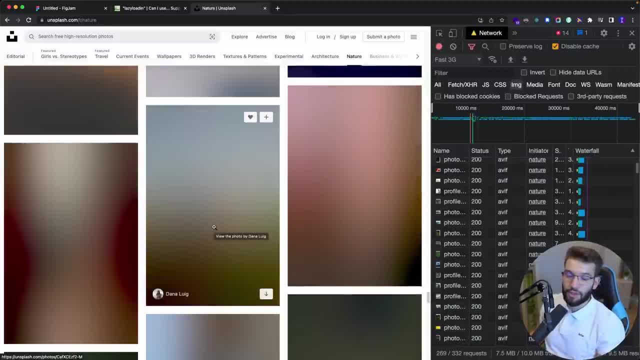 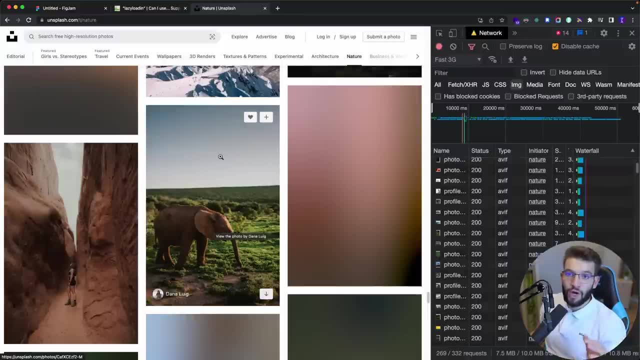 So this is the perfect image optimization technique that in Splash uses, And we try to use or actually reverse engineer how Splash works and try to implement that on our own application, And we're going to, of course, use React with TypeScript JavaScript. 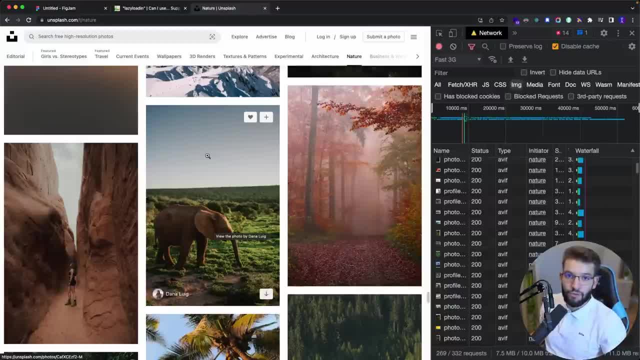 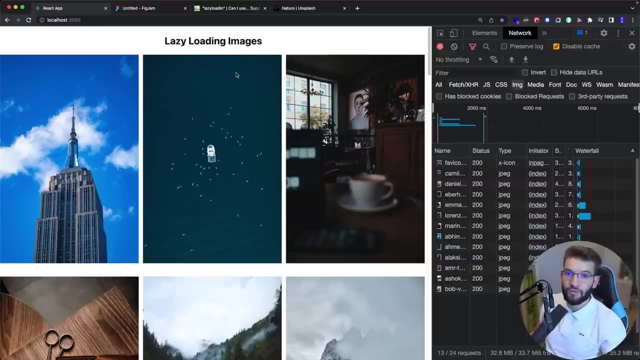 And you can use that with regular JavaScript if you want, But we're going to use React for this particular video, All right. So the first technique I'm going to be trying in here is actually using the native lazy loading feature provided by the browser and the new HTML standards. 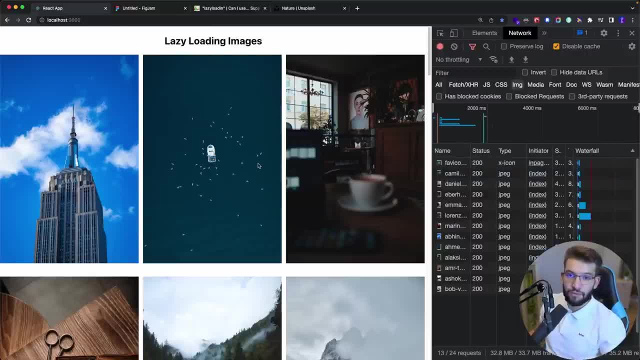 So there is actually a lazy loading feature for images and web frames, But I'm going to talk only about images, this particular video. So for images, browsers like Chrome, Safari and Firefox- like the newest versions, of course- actually support lazy loading by just providing an attribute. 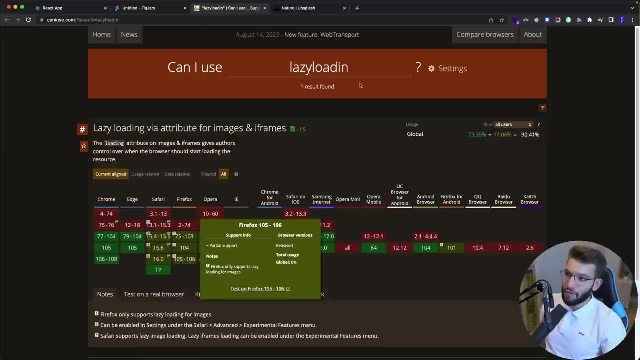 to the actual image. So by looking at the- can I use web page in here for lazy loading- you're going to find what are the support browsers. So if you look at Chrome, it started from 77 version to the current versions. There is Firefox. 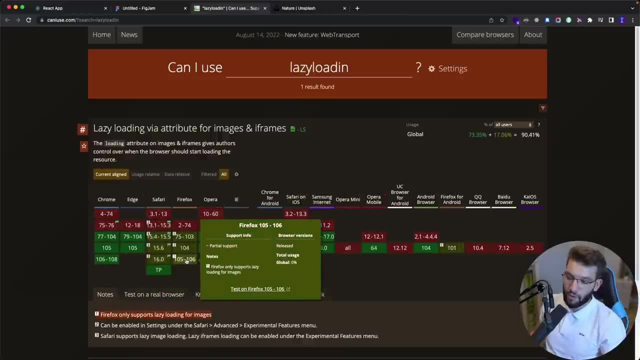 It has partial support because it doesn't have support for web frames or it doesn't really work for those, And Safari as well has some issues in partial support, So it's not that widely supported. It's not 100% going to work fine across all browsers. 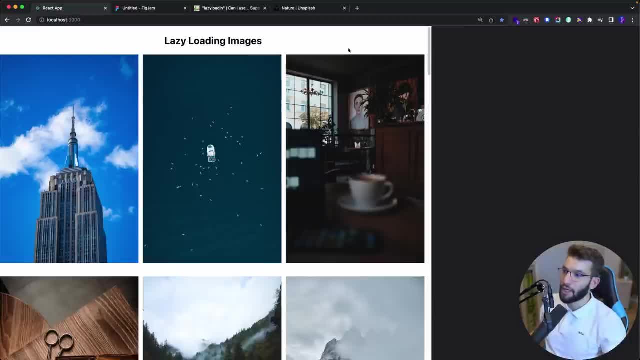 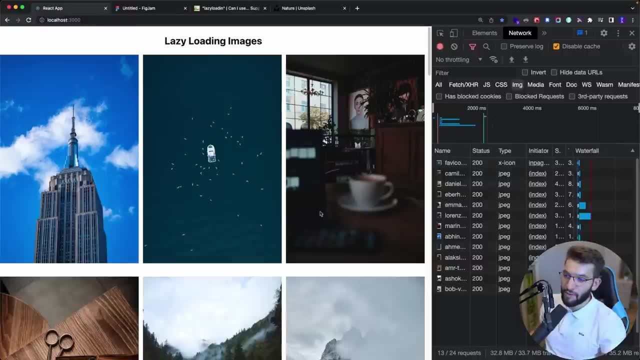 So that's quite an issue. But if you go to Chrome it works perfectly. So, for example, in our web page in here I'm going to look like: as soon as the web page actually loads, it's going to load only the set of images. 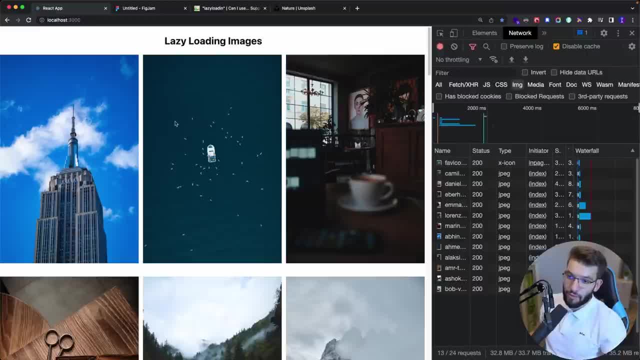 that are going to be visible to the user on the viewport. So in the viewport in here we're going to have only six images visible, or just a set of images, because it has some threshold. So only 13 images are loaded in here because I have a filter on images. 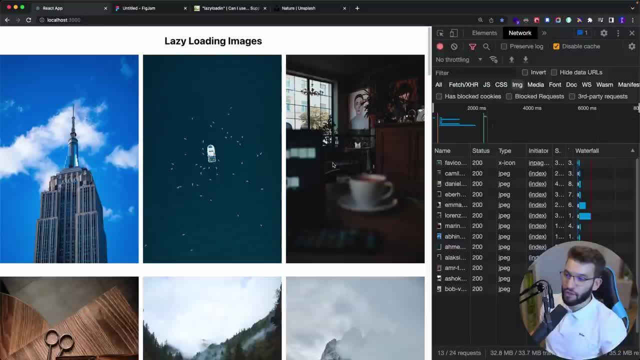 And it got like 30 images on the whole web page. Now lazy loading. I have lazy loading here. If I lazy load it, as you see, it loads more And I can just go and include a console for you to see. 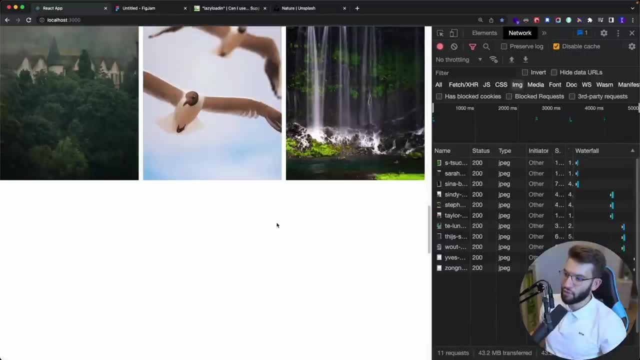 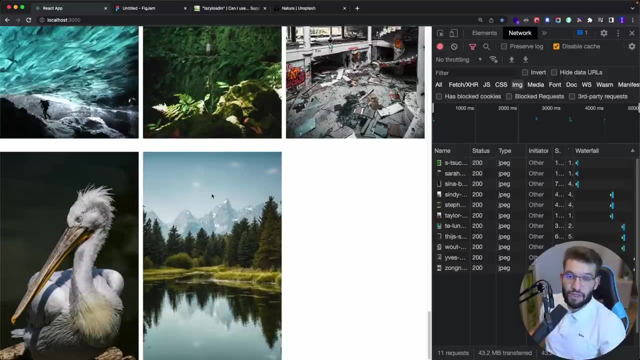 So as I scroll, it's going to load more images And as the user approach, the other images, like: eventually, all the images are going to be loaded in here. And that's exactly what's happening, And this is really fun. It works really well. 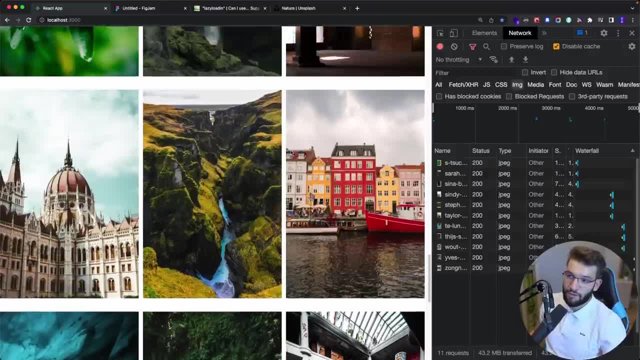 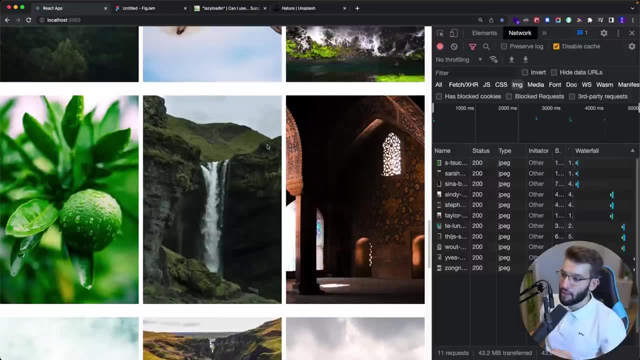 It loads images, It saves you data, It saves network bandwidth. If the user is not actually viewing that image, why would you need to actually load that image at all? So that's lazy. loading is perfect And the way actually to implement this. 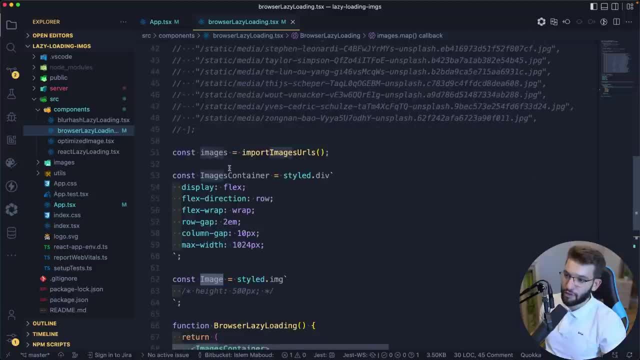 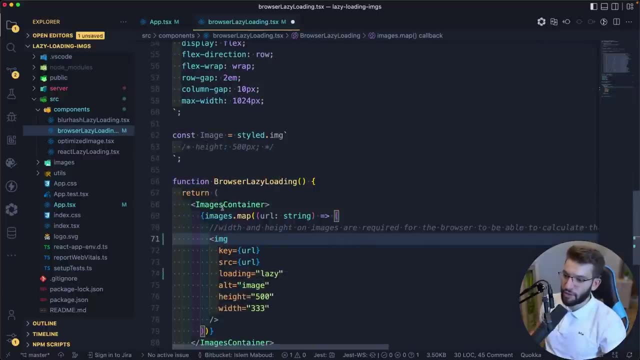 is super, super easy. So on the image: in fact this is just a regular image, because what I'm having in here is just a regular image styled image, So you can go in and replace this with an image in here. So this is a regular HTML image element in here. 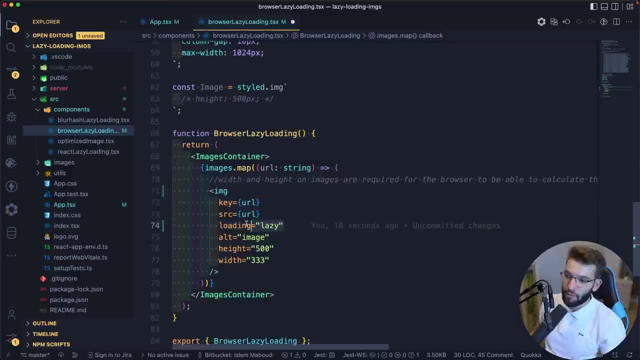 And it has everything, a key and everything, And the most important prop or attribute that you need to add is the loading attributes, with either lazy, which is lazy loading, or eager, which is by default, which means load all images when the web page loads, which. 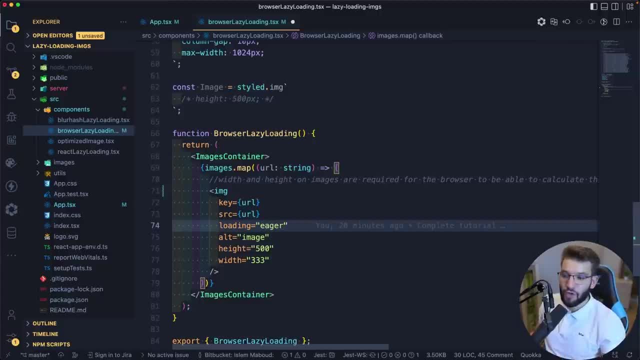 is pretty bad experience, of course, because it's going to give the user the impression that, oh, the web page is not loaded yet because you got tons and tons of images that you're trying to load, Even though you've got 100 images. 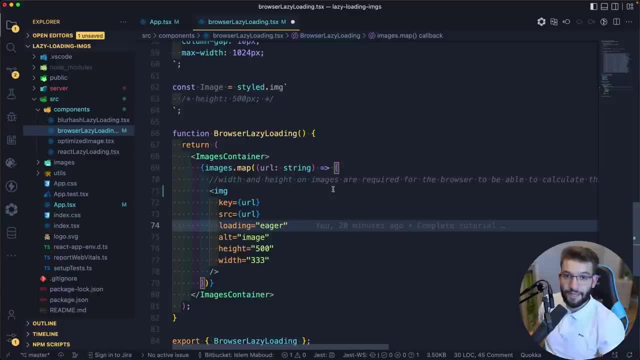 and you're not, of course, going to reach 100 images because you haven't scrolled just yet, which is quite bad as of a user experience perspective. So that's really not good. So using lazy in here will do the job and will do it perfectly. 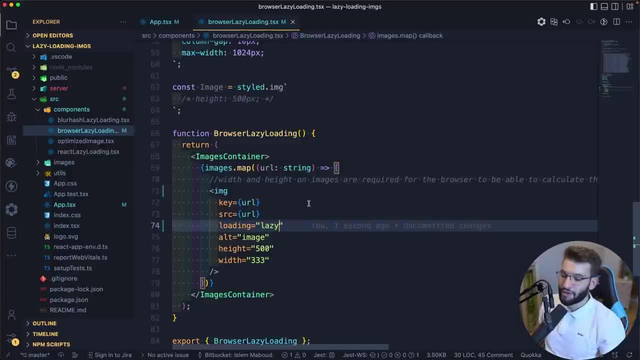 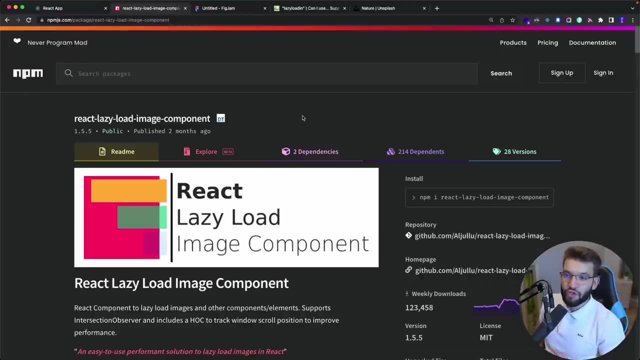 And that will use the native feature. But still the native feature is not really that perfect. Plus, it doesn't have that best experience of what Unsplash actually provides. Now the second best approach you can do to lazy load images and have a great user experience: 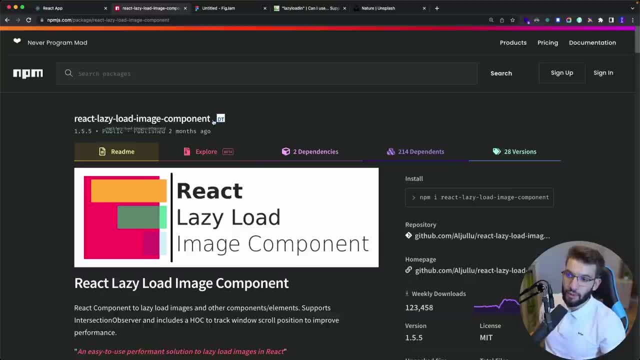 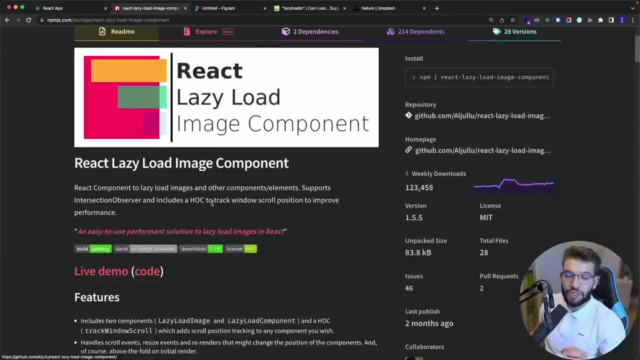 is using a component called React Lazy Load Image Component, And this component actually provides you with a real user experience because it gives you the state of image, whether it's loaded or not, And you can apply some effects telling the user if the image is fully loaded or not. 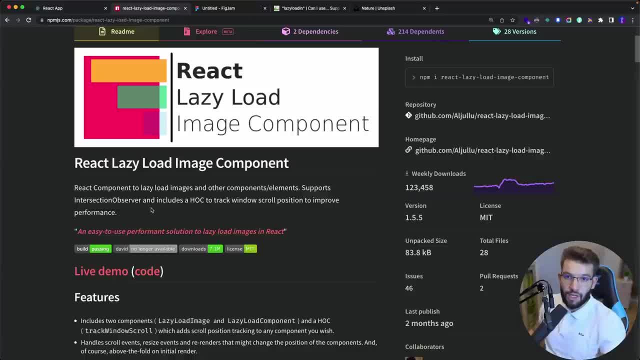 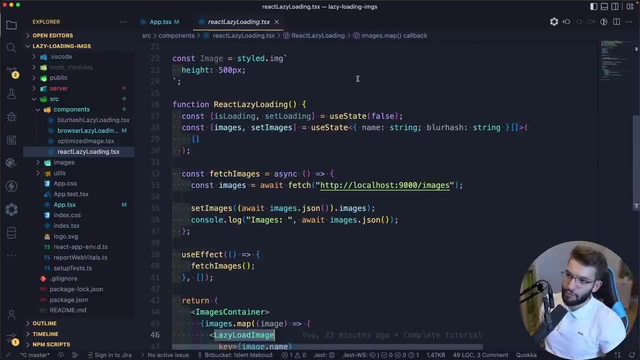 You can do black and white or blur the image into that image that is fully loaded by the browser. All right, so if we're using the component here, we just import the lazy load image component, which is from the library, of course. 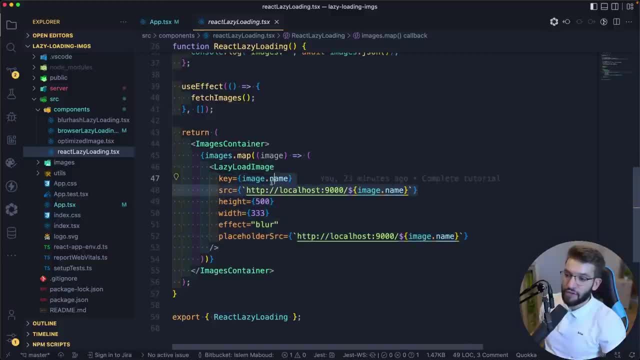 And you just use that And, of course, you're going to give it a key. You're going to give it the SRC of the actual image, height and width, because it has to determine the height before the image actually rendered, so you can have 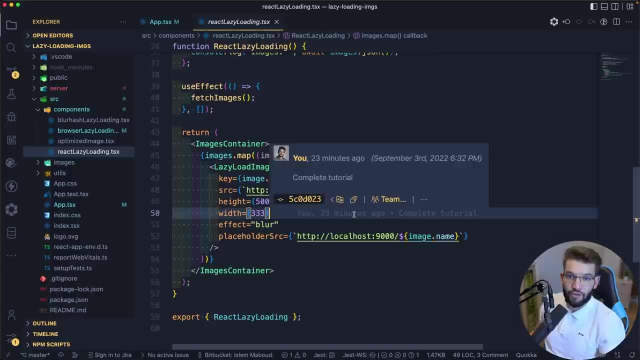 like an awesome placeholder for the user before the actual image is loading. And you've got some effect in here. So what effect do you want to apply? So you can have blur or black and white or everything. I think blur is good enough for this. 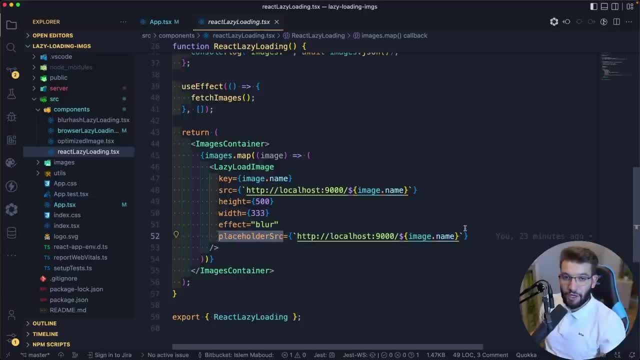 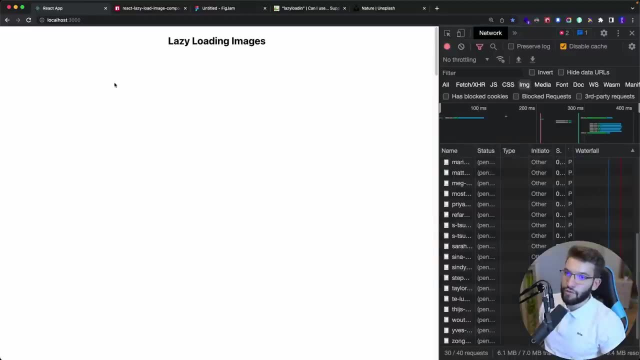 And you've got a placeholder SRC, so which image you want to show in place of that current image that's still loading before it actually loads. So if you go to our application in here and refresh using the new component, as you can see in here, it provides some awesome blurriness. 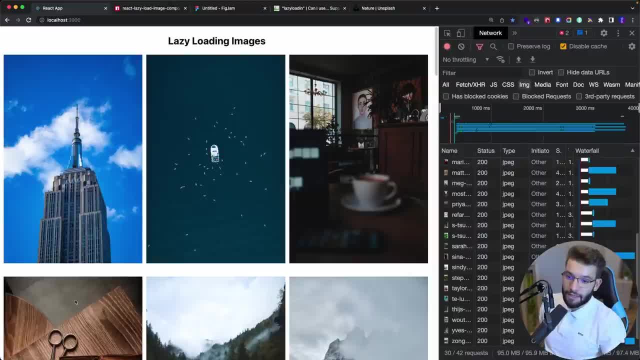 effect. So before it loads, before it actually fully loads, it does some blurring effect in here And as well as the effect alongside that, of course, it's going to still do the lazy loading thing. So when the user scrolls into the images, 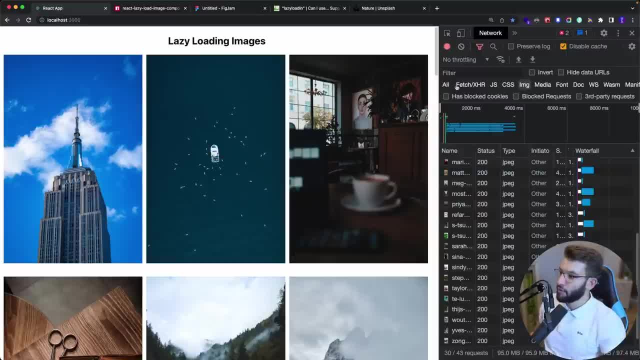 it's going to load that images. So that's what lazy loading is. So, for example, you've got a set of images loaded in here first. Now I'm going to go and scroll As you can see. the other image is going to be loaded. 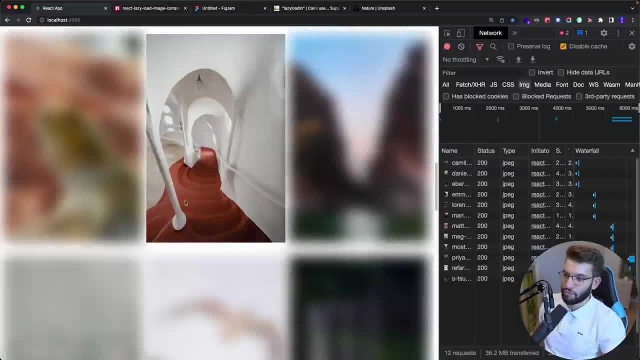 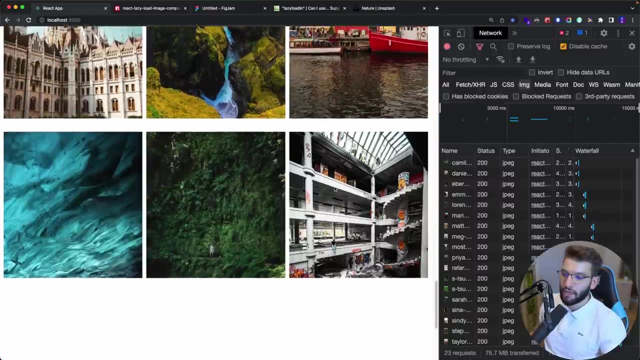 It's going to have the awesome blur effect. So, as you can clearly see, it works really well with this really perfect blur effect. So that tells the actual user: oh, you got some image loading, So just hang on there and let the image load. 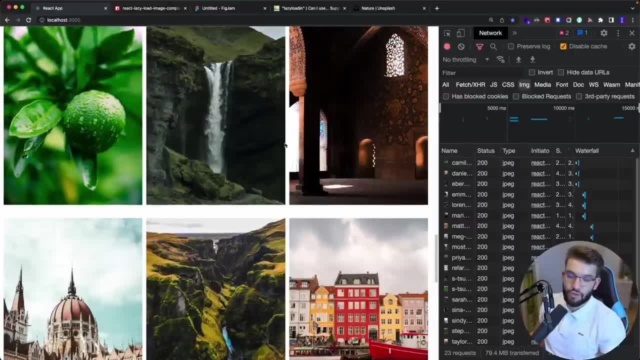 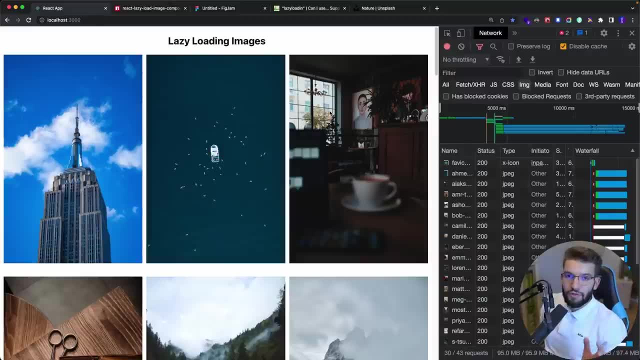 So just wait a couple of seconds because you got a really bad network connection or the server is not responding in time or something. So that's exactly what's happening in that case scenario. So as far as this solution and using this lazy loading component with this awesome blur effect, it's actually good. 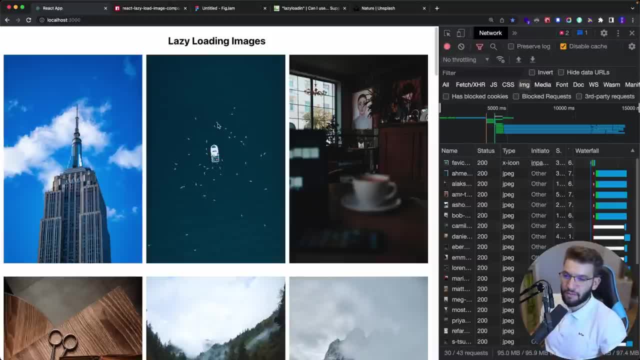 But it's not that good. In fact, it's not really perfect And it doesn't provide that really well awesome user experience as we wanted to have on InSplash. So I'm just going to give you one reason why this approach is not. 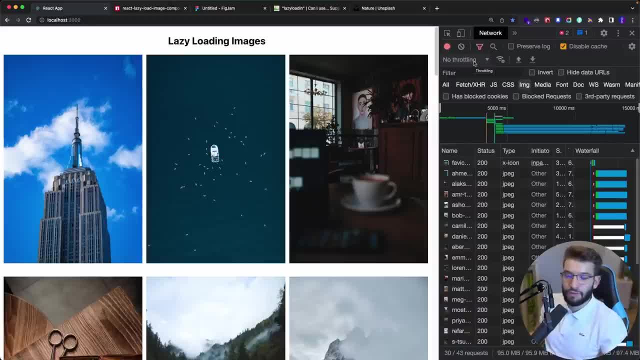 really that perfect. You may still use it. Of course, you can just provide some tricks around it and just try to provide some hacks around it to make it work perfectly, But it's still not going to be that perfect. So if I go to Throttle in here, I'm 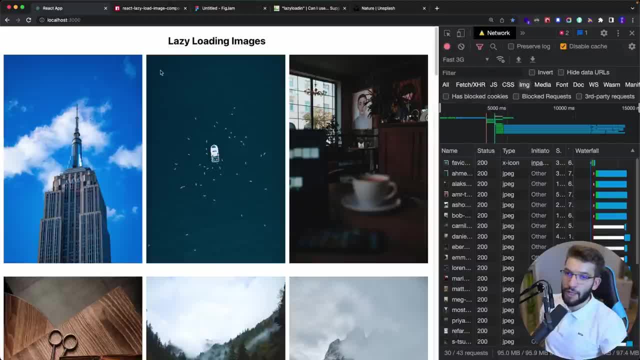 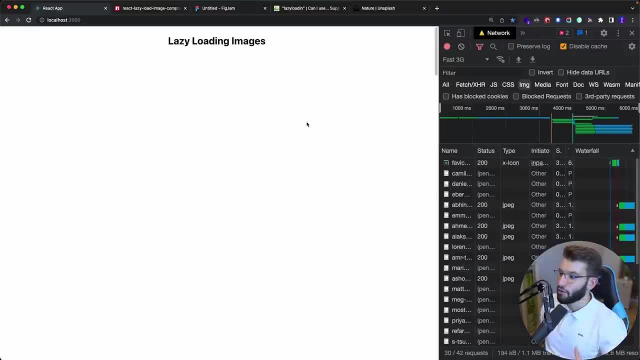 going to throttle the network to fast 3G, right, And so I'm going to go ahead and try to do this Like fast 3G. I'm going to refresh the web page in here and see how fast or how the loading experience for a very 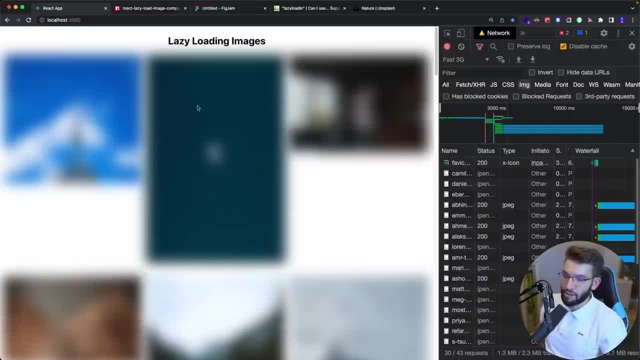 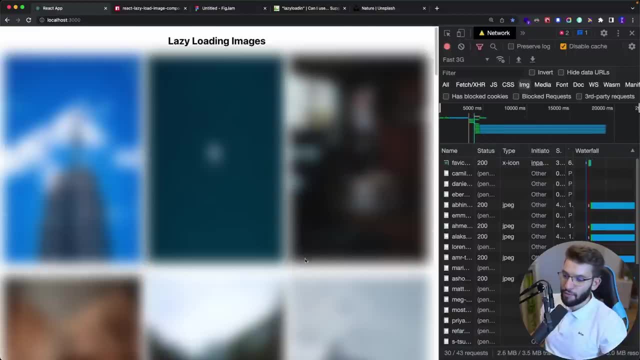 bad network in here. So how is it going to be excruciating? It shows you that the images are not fully loaded, So the blurriness is not affected, only on the image. So it tells you that you got this image loading kind. 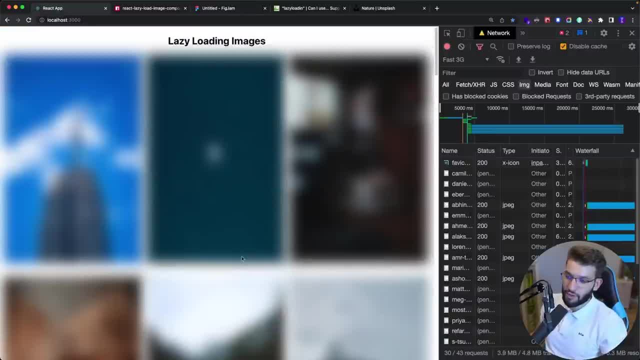 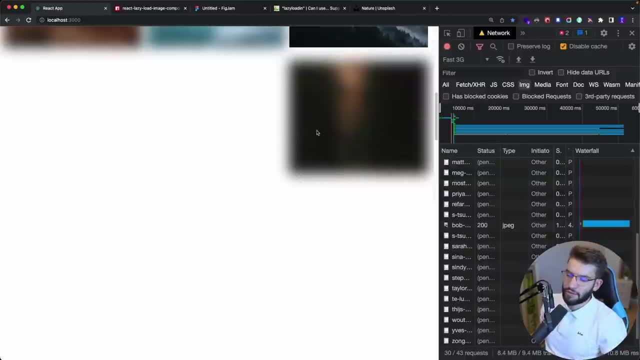 of experience And once, of course, some pixels of the image loads are obviously going to have this awesome blur effects, But before that, you're going to have this really good blur effect And yeah, so it's not really that perfect. 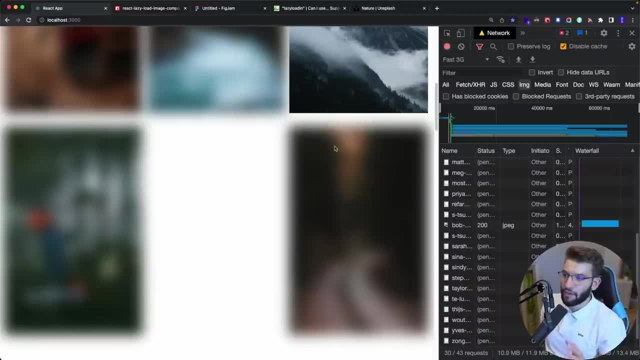 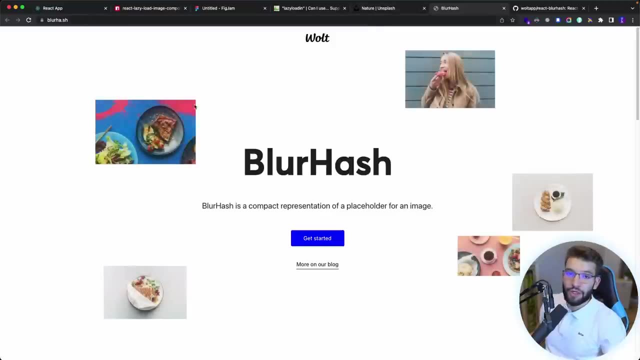 So you see the actual image loading. I don't actually like it that much So the third approach that I find is actually the perfect approach that simulates the same way nSplash is implementing their image optimization and lazy loading and having all this awesome blurred placeholders and everything. 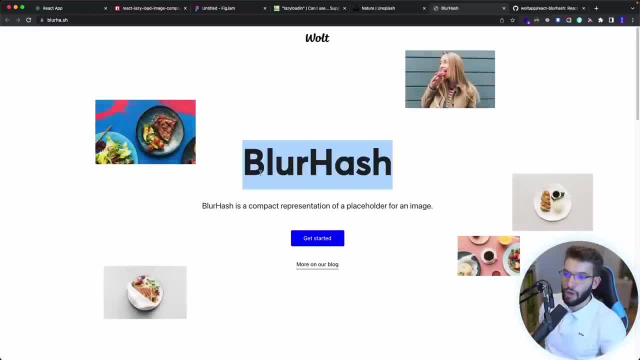 is using this BlurHash library And it's really really awesome library. It's available in all languages pretty much And the library will work. But it's actually giving an image And it gives you kind of like a hash that displays its placeholder. 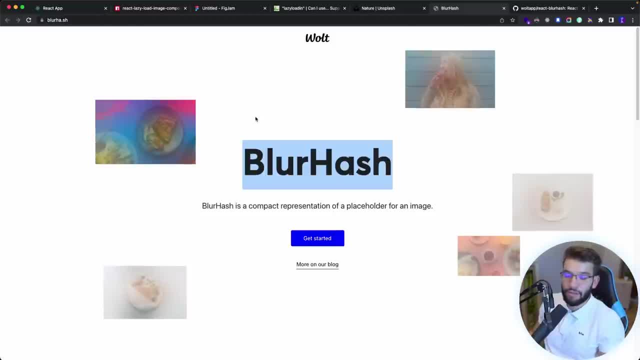 And it looks amazing And that's exactly what nSplash is doing. So as far as I like reverse engineered, it looks identical to nSplash's stuff, But maybe nSplash is providing or doing like implementing their own algorithm or something like this. 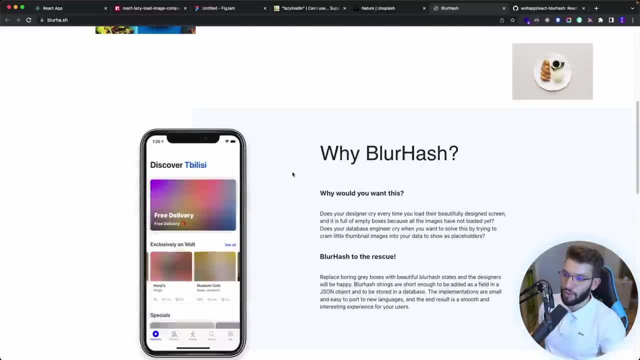 But this is more of like the best solution I can go through here. So of course this is an open source. It's not like a server or something, And this is what it does in here You give it just an image, gives you a hash. 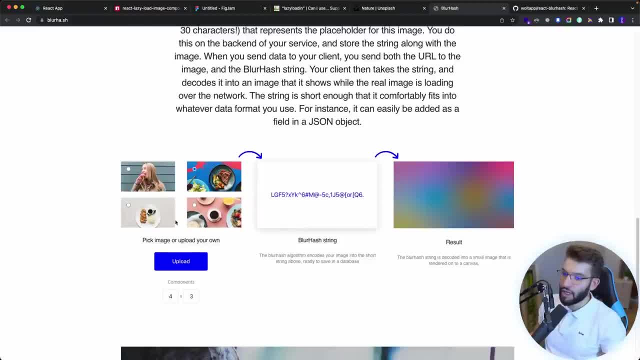 And you can just go ahead and render that hash And this is the result that you're going to get. So any image in here. of course you're going to have a different hash And of course you can get this blurred image. 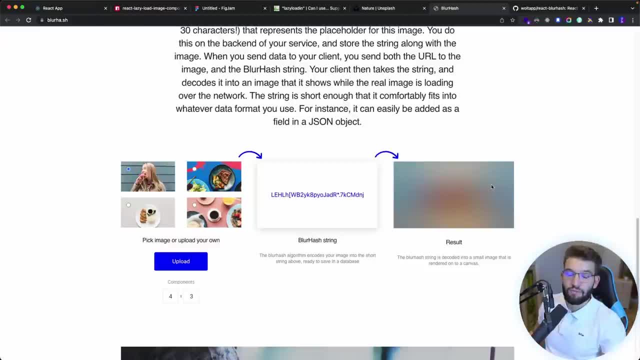 And, of course, what you can do is display this blurred image before the actual image is fully loaded. So the user knows: oh, I got this blurred thing And I'm looking into its blurred image, obviously, But I can clearly see what the image would. 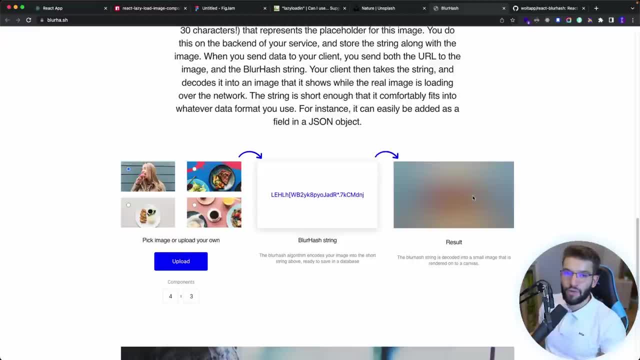 look like after it loads. So the user knows: oh, I'm just going to wait for this image to load And this is a lot better. This is a lot better user experience Plus, you're not going to have this reflow issue. 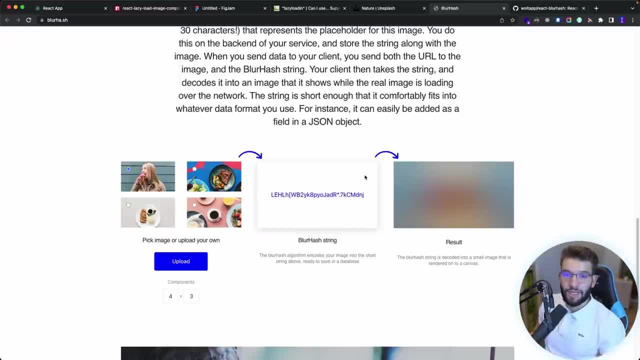 If you're not familiar with reflow issue, you can google it out. But it's more of like overflow issue with CSS and everything to have it work properly before the images are loaded and taking their original positions and places and everything. And the great news here: React has this BlurHash library. 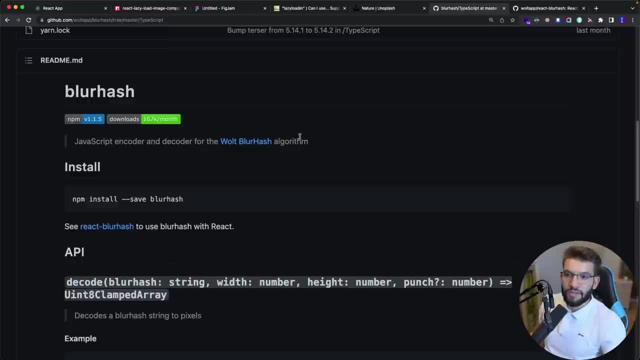 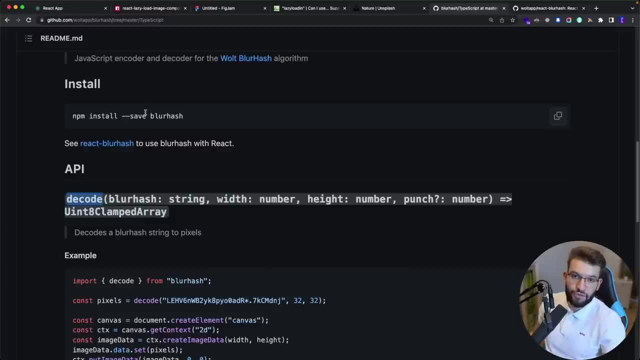 And it has it in an easy, simple way that you can go ahead and implement. So, in a basic sense, how BlurHash actually works is you can have two methods in here: a decode method with BlurHash that has been generated by BlurHash itself. 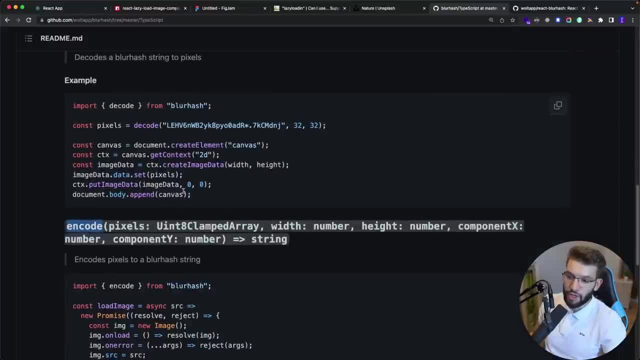 And you've got encode to encode the pixels into a BlurHash And obviously the BlurHash is going to be more of like very small string in here. So, compared to if you do it to base64, some people say, oh, I'm going to do it in base64. 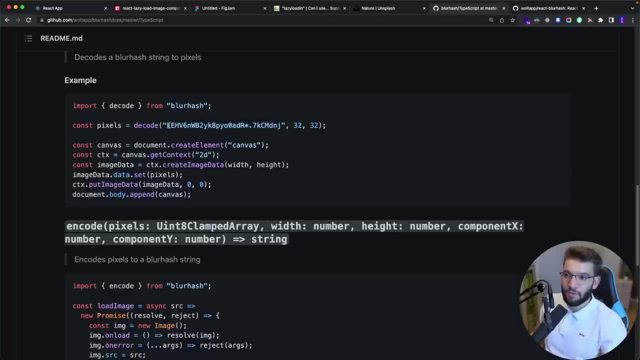 Yes, you can fully do it in base64.. But if you have like really large image and you can double scale it, of course, But you still got problems with this because the base64 is like more than actually 100 characters, right, 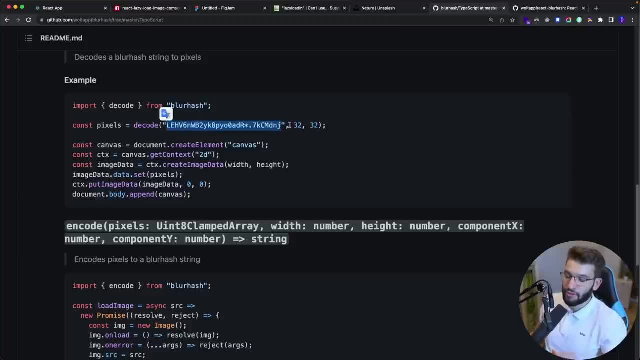 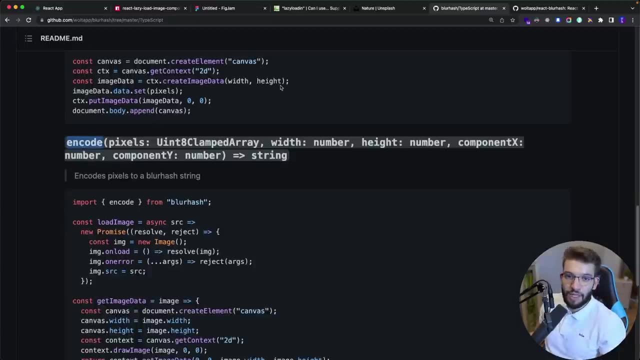 But this one is, like you know, 20 characters or 30 characters- It's a lot smaller, OK- And the step that you need to go through is actually encoding the image, So this could be done literally anywhere, depending on your application. 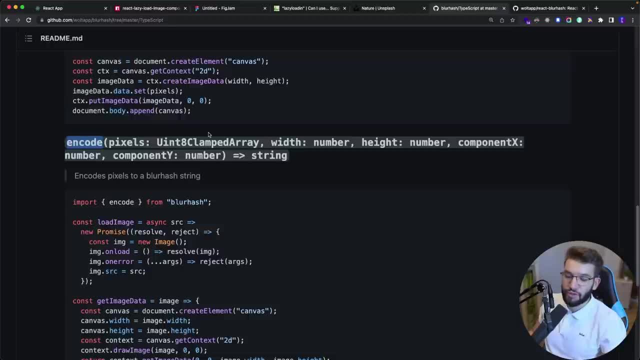 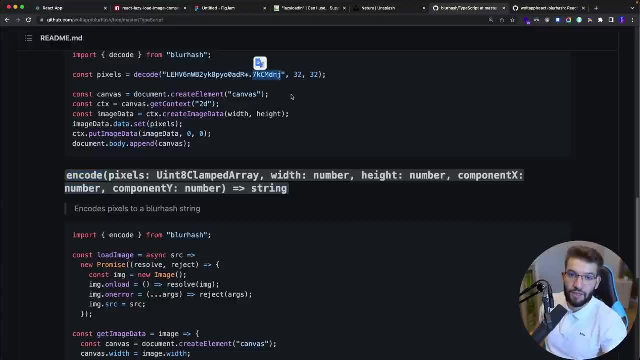 But in our case in here I did them actually and put them in a JSON, So just to simulate the server kind of thing. And obviously what you want to do with these hashes is actually store them alongside the image paths on your database or something, because there 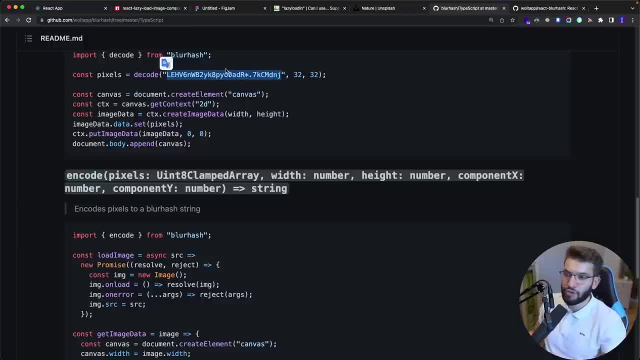 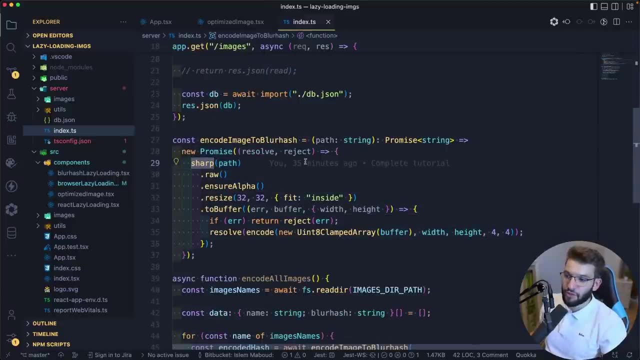 are very small strings in here And every single time you return an image, you're going to return that string right along with it, And that's exactly what I did. I just used this include thing, I used sharp and everything. You can check out the code source or the source code. 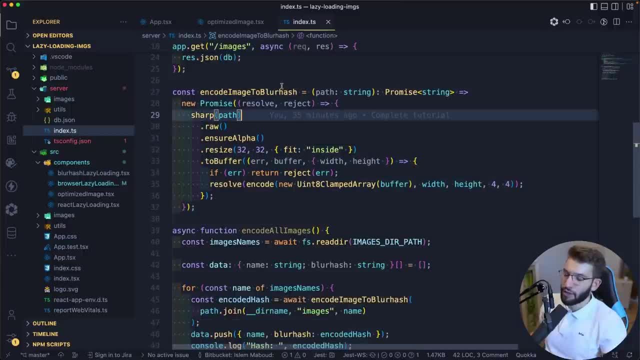 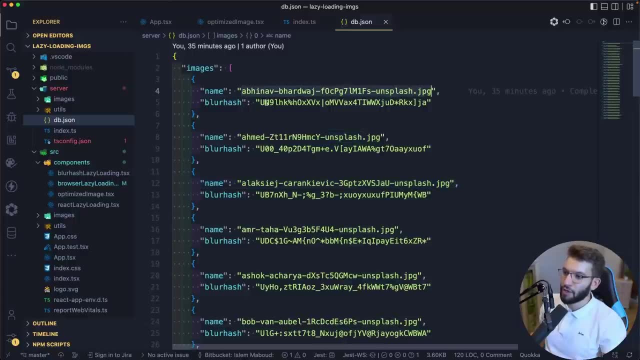 in my GitHub in here and how I did that, like all the encoding process and everything. And after I encoded this, I put it onto a JSON And that's what I did. So I put the image name and I put alongside of it. 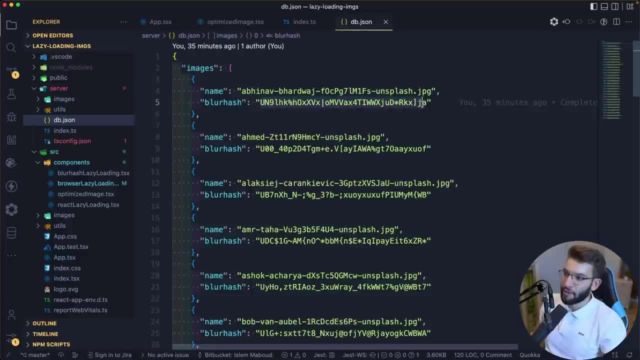 like the blur hash of this particular image. And that is it. It's just that simple. And every single time the user requests the images, I'm going to return that blur hash alongside of it to make it work perfectly. And the result of displaying the blur hash: 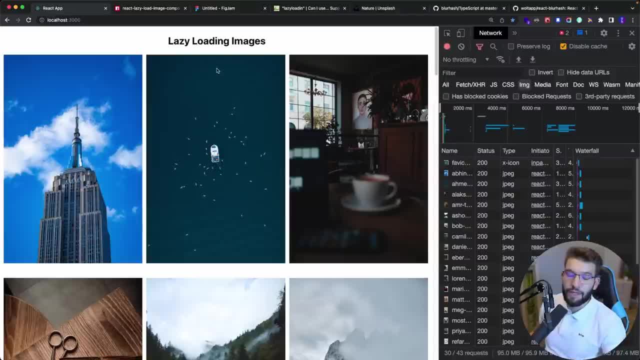 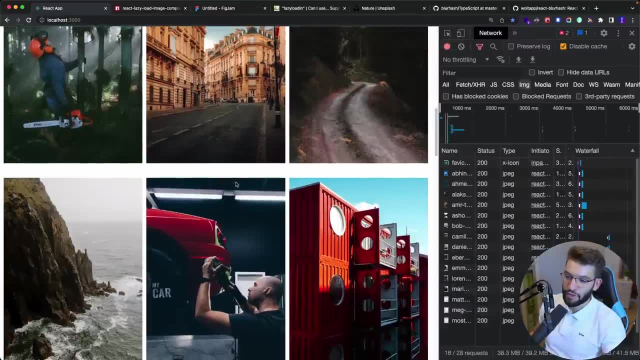 placeholder when the actual image is still loading is actually amazing. So, for example, if you're refreshing here, that's the actual placeholder of blur hash And as you scroll it's going to steal the blur hash And as soon as the image loads, the blur hash. 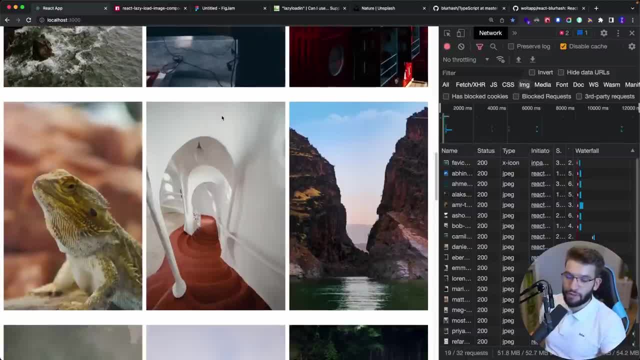 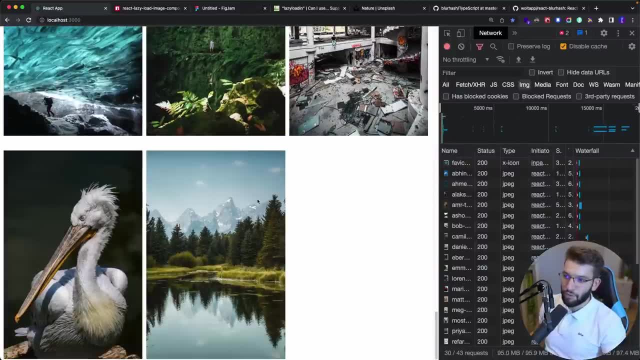 is going to be gone, obviously because we have some logic in the code doing that. So that's actually working absolutely fine And, as you can see, it looks amazing. You can immediately see what the blur hash version does Now, for example, if you introduce some throttling. 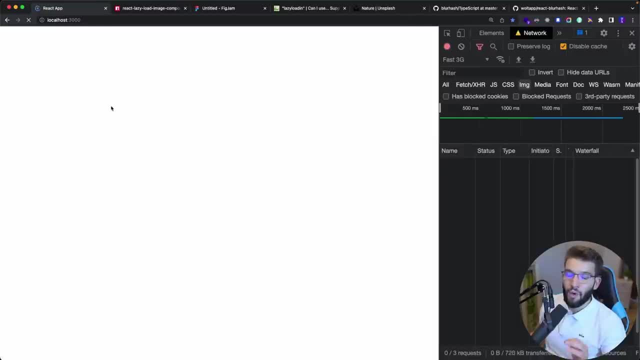 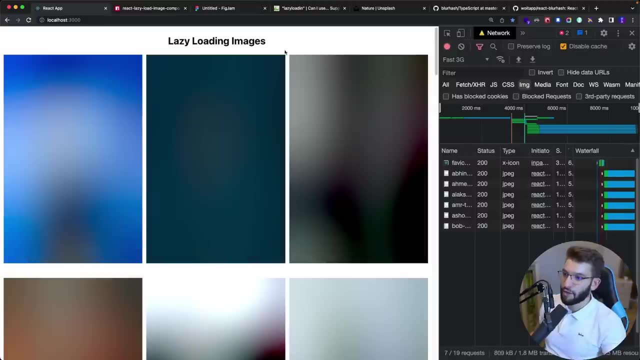 in here for fast 3G refresh the web page. we're going to see a way much better experience, as we did before with the lazy load components image that we've tried, like the React component thing. So, as you can see, placeholder in here is looking amazing. 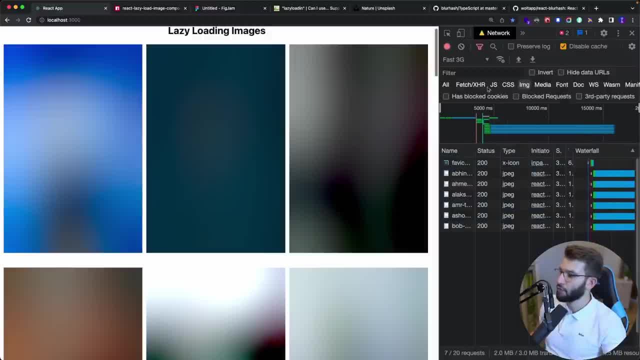 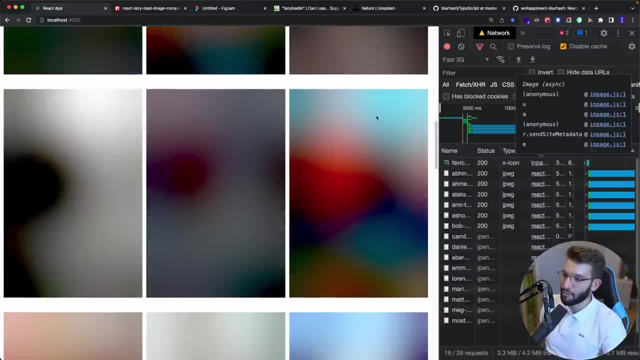 The images, all of them are still loading because you got a pretty awful network connection in here And we got the placeholders. We know exactly what's happening. We can see all the placeholder in here. We can see the blurriness of the image. 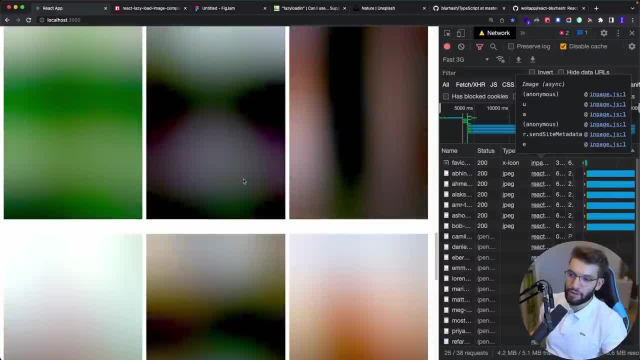 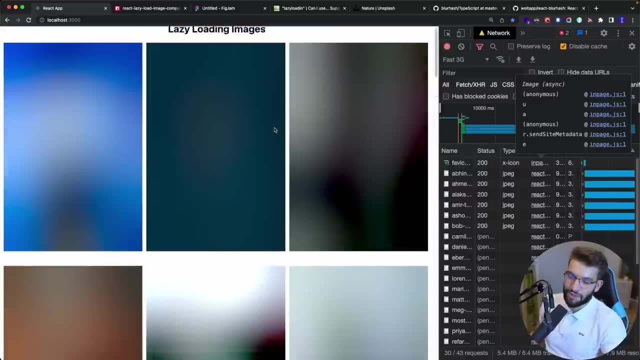 And we can see some sort of content of the image And we can know: oh, the image is loading. Yes, I'm going to use here, I'm going to just sit down, I'm going in here and wait. So maybe go ahead and grab a copy, because it got like a really bad 3G. 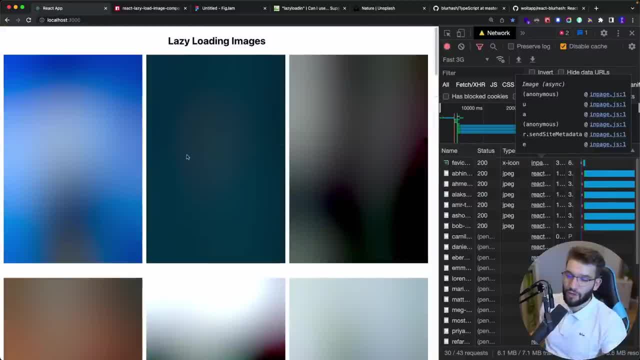 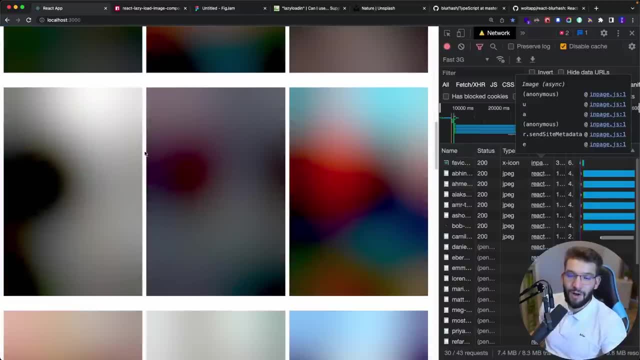 network or something of that sort, But it works perfectly, a lot better than before And it doesn't really cost that much. I mean, I don't know how I didn't know about this before, But that's a crazy awesome solution. 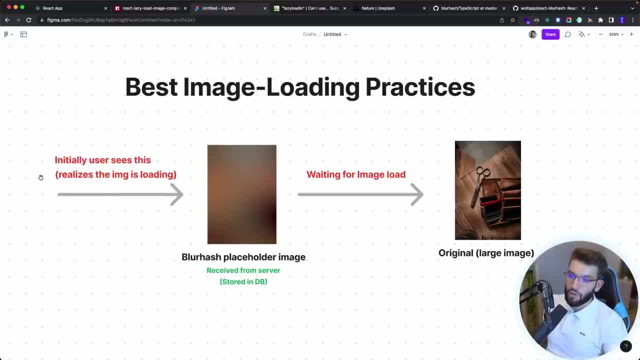 And if you're wondering of how the blur hash is actually working or the technique we're using in here and what Splash is actually using. so basically, first what it does: it actually loads and puts the placeholder like the blur hash placeholder here, before the actual image is loaded. 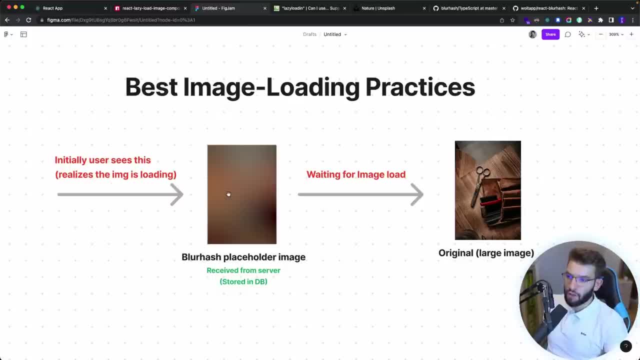 So it just puts that and renders that. So the user would tell: oh, I know This is an image actually loading, So I'm just going to wait for it And, of course, if the image takes forever, you've got this placeholder. 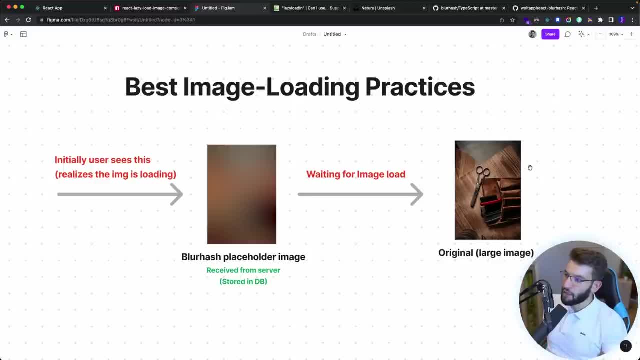 And the user still waits, like whatever. But once the image is loaded it's going to be replaced. So this is going to be completely ditched off, removed from the DOM, And this will be completely replaced with the original image. And the image is fully loaded. 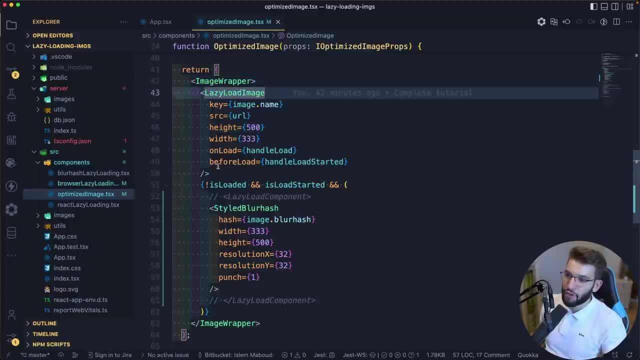 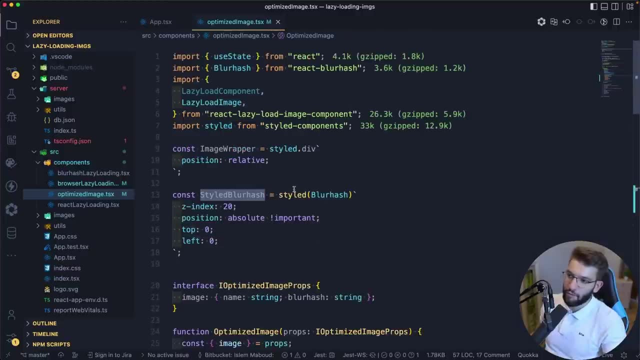 And, of course, for the actual front-end coding. here we're simply just putting the image in here, putting the lazy load image in here. Now, of course it's going to be lazy loaded every single time we scroll. The style blur hash in here. of course, I just put a style. 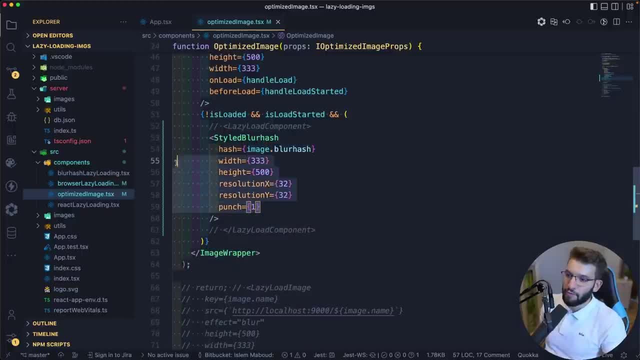 to have some CSS in order to make it work properly, And we just display that before the actual image is fully loaded, So this will look absolutely amazing.